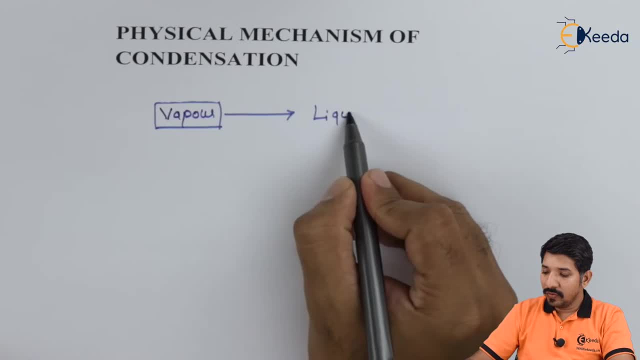 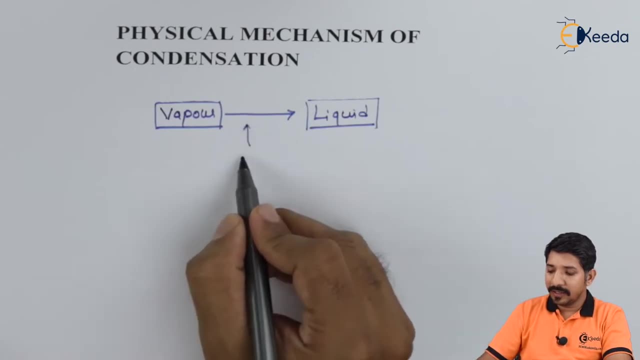 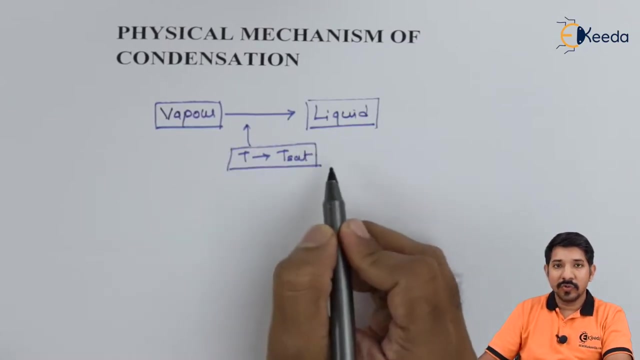 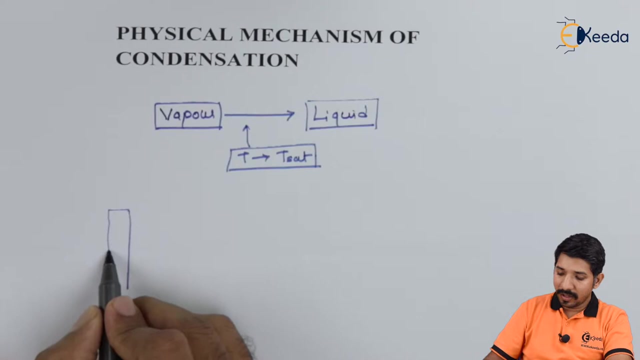 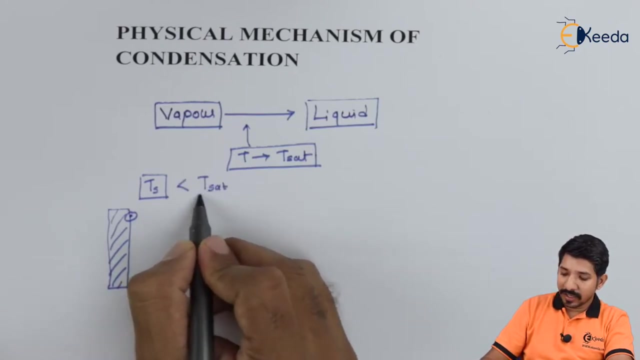 The condensation is nothing but the change of vapor to liquid. Now, in this process, the temperature is reached to a saturation temperature. So basically we can take an example. Let us consider an example. A surface is, let's say, the temperature. is the temperature of the surface is kept below the saturation temperature corresponding. 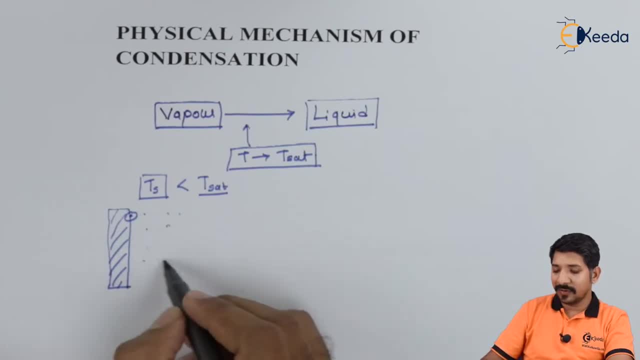 to the pressure of a given fluid which is there around it. If that is happening, what may occur? that, due to this, a liquid will get condensate, or a small droplet may get condensate over a surface. Whatever may be the condition of the condensation, the reason is simply the surface temperature. 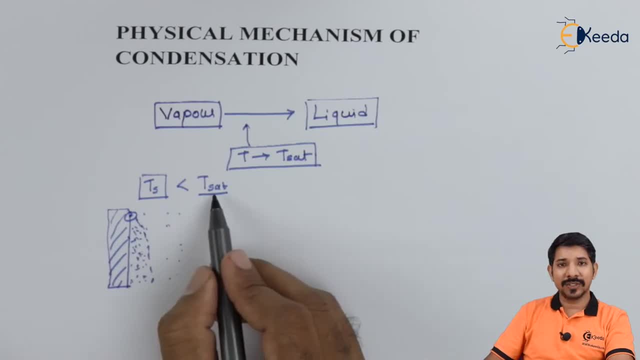 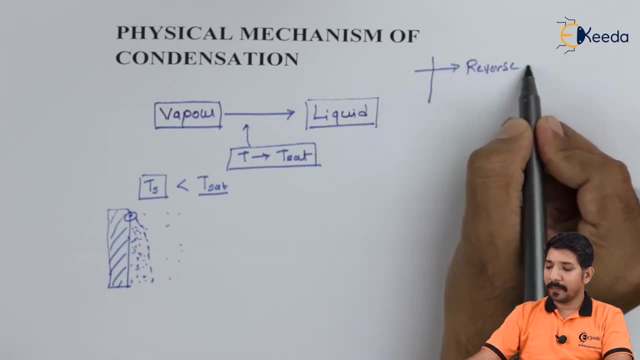 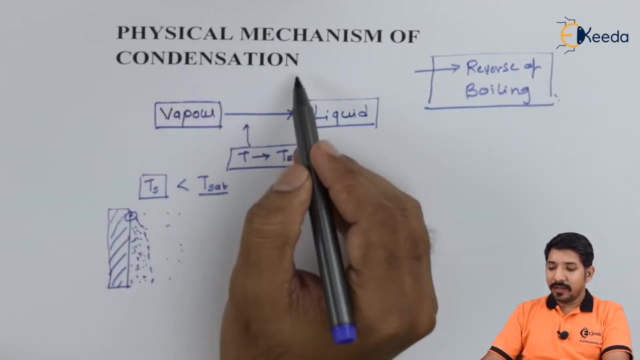 of the given wall is less than the saturation temperature. So what we can say is: this is nothing but a reverse of boiling itself. So the basic definition of condensation is nothing but where, as we have seen for boiling, we have discharging of the condensation, and this is 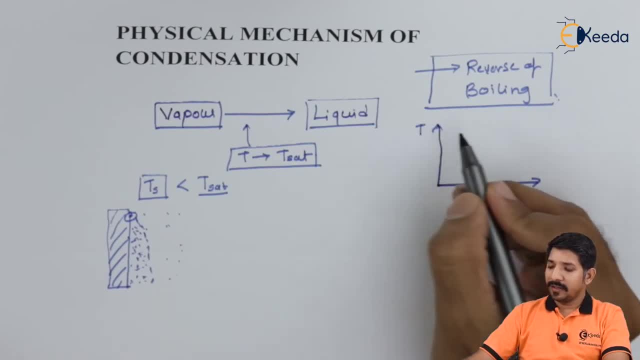 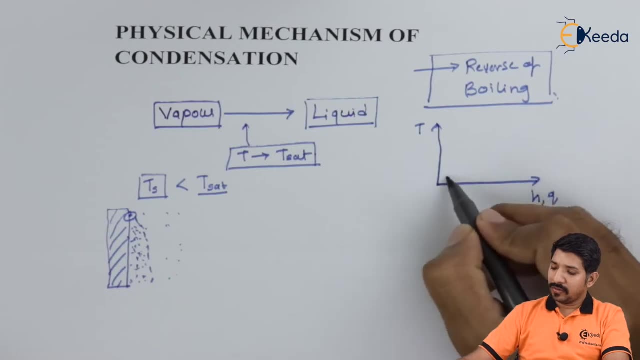 what it means. So we will see that what we are trying to do is that we have taken an drawn this diagram previously, where on Y axis we have temperature and on X axis we have H or, let's say, Q. So if I keep on increasing the value of H or Q, the temperature will keep. 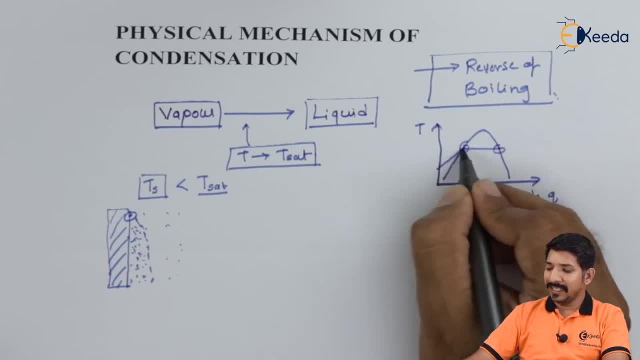 on increase till it reach to a latent heat or a saturation temperature. So after the saturation temperature, once it reach to a saturation temperature, there will no longer be any increase in temperature, even if I am adding some heat. Now what is this heat? they call, as they call this, as a latent heat, and after that again, if I keep on increasing, 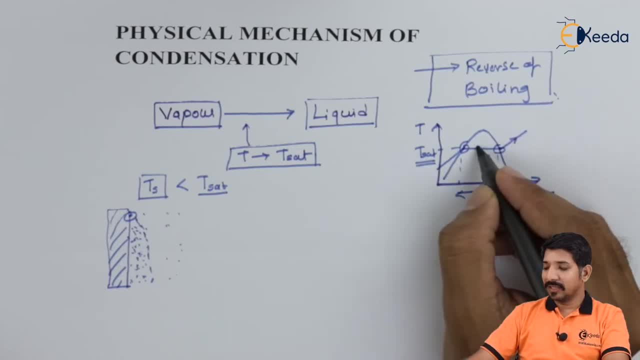 the value of Q, my temperature will start increasing. Now, this was the case of boiling. Now, this was the case of boiling In case of condensation. we will start from this point. So, basically, the vapor we will start is kept at this temperature, will keep on reducing heat and till it reaches to certain point.